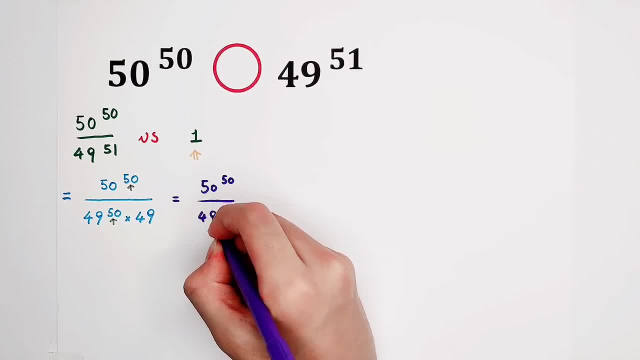 It is 50 to the power of 50, divided by 49 to the power of 50. This denominator, 49 to the power of 50, belongs to our numerator, And then I'm going to separate This 49,. let it alone. let it be alone a good idea. 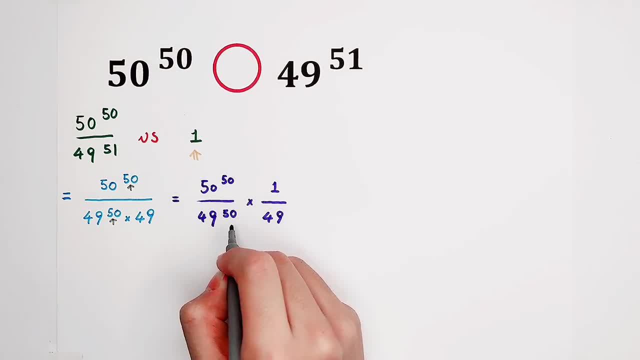 So now 50,, 50,. they have the same exponent. We can take out this exponent. Therefore, it is 50 over 49, and then also our 50, then times 49.. Oh sorry, 1 over 49.. 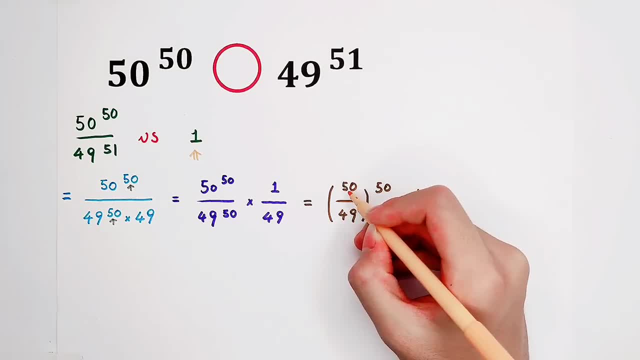 This fraction inside the bracket. it is 50 over 49.. 50 and 49, they have a special relationship. That is, 50 is 1 more than 49. So it can be written as 1 plus 49.. 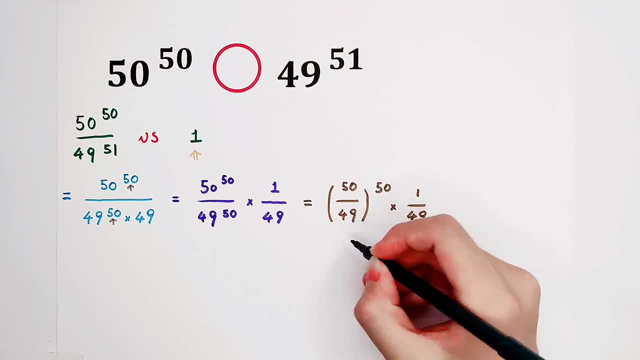 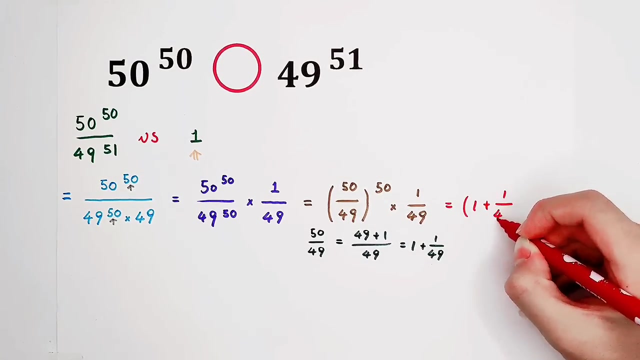 So therefore it is this: 50 over 49.. It is 49 plus 1 over 49.. So then it is 1 plus 1 over 49. Therefore it is 1 plus 1 over 49, then also our 50, times 1 over 49.. 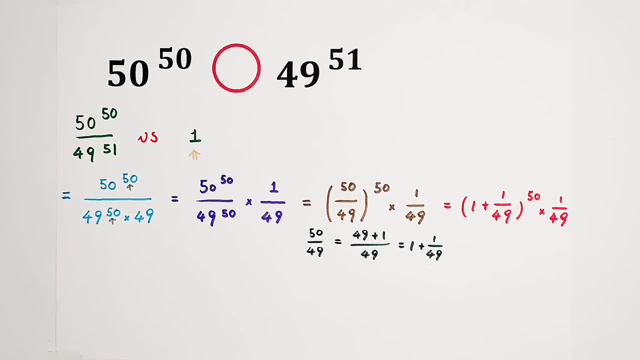 To tell the truth, a problem is coming. We meet a problem. What is the problem? Please have a look at this section: 1 plus 1 over 49, also power 50.. What is the problem? The base or the exponent? 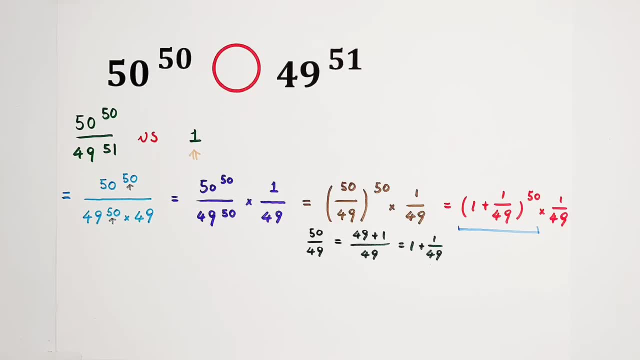 Maybe you want to say the base, because the base is so complicated. However, the answer is the exponent. The exponent 50 has a problem, A bad-looking term. we don't like its form. We always like 1 plus 1 over n. also power of n. 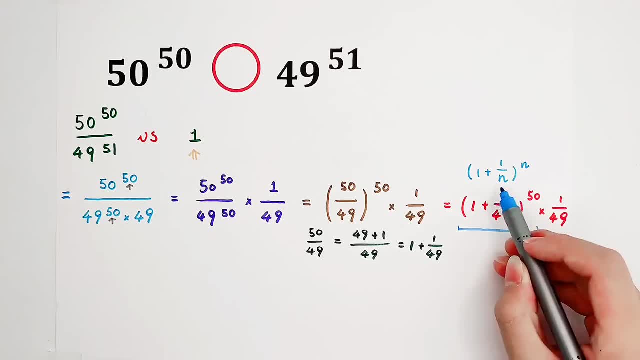 This form. However, if we substitute 49 for n, the exponent is not 49, it's 50. So what's the problem? The exponent. So how can we deal with the exponent? I have a trick. Look, we can separate 49 from this 50.. 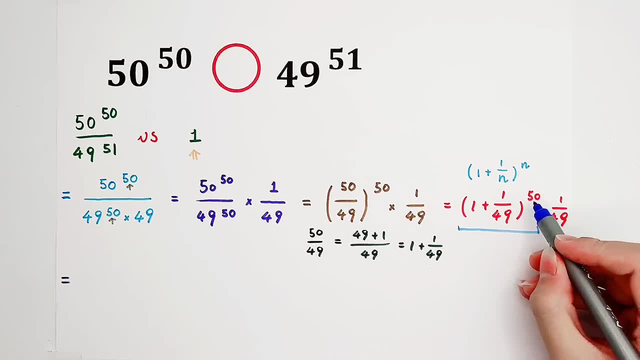 That means I can consider 50,, 49 plus 1.. So it can be written as it is only equal to 1 plus 49,, also power 49, and then times 1 plus 1 over 49, and then times 1 over 49,, don't forget. 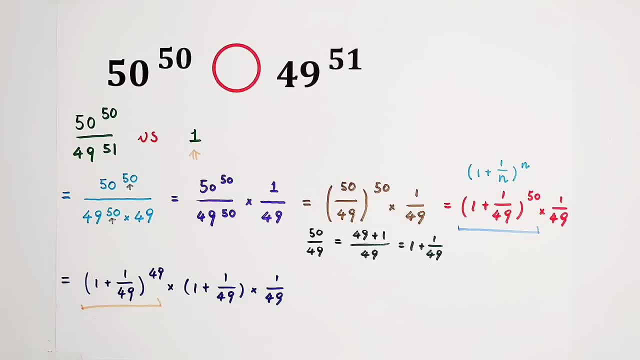 Now the problem is this guy: 1 plus 1 over 49, also power 49. It has the form 1 plus 1 over n, also power n. So then I don't know if you've heard the Euler's number E. 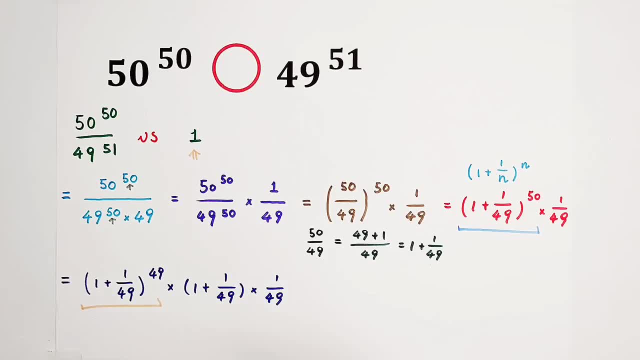 If not, learn it now. The definition of Euler's number E. it is the limit. I'm going to write it here. okay, The limit of 1 plus 1 over 49.. Plus 1 over n, also power of n. 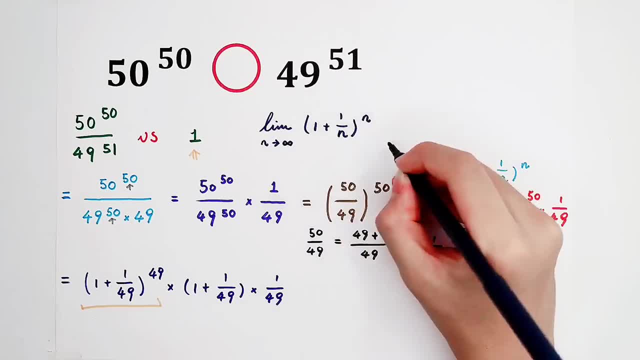 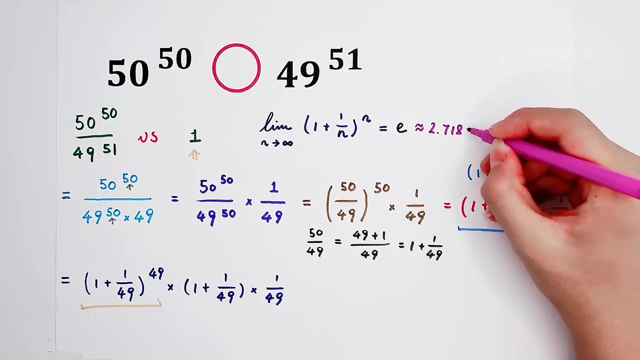 When n tends to infinity, The answer is E. What's that? It's a letter. Now, it's a number. actually, What does it approximately equal to? It is approximately equal to 2.71828.. 1828459045, and so on. 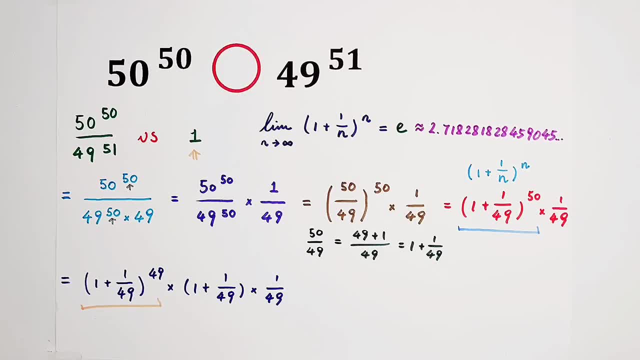 It is irrational. It is so complicated For this question. this method is a piece of cake. It is very easy to understand Why. Please have a look. E is approximately equal to 2.718.. It is, of course, smaller than 3.. 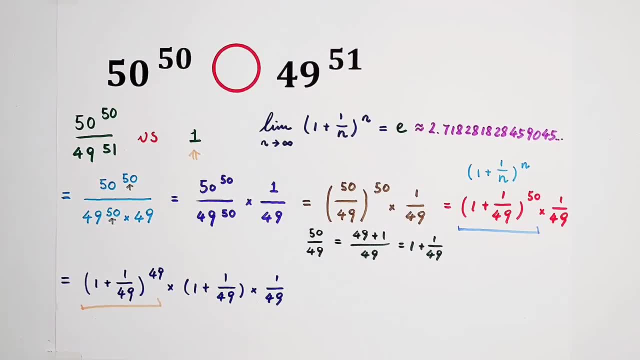 That's the only thing which is important: It is smaller than 3.. Whatever n is, 1 plus 1 over n- also power of n- it is always, always, always, always, always, always smaller than 3.. 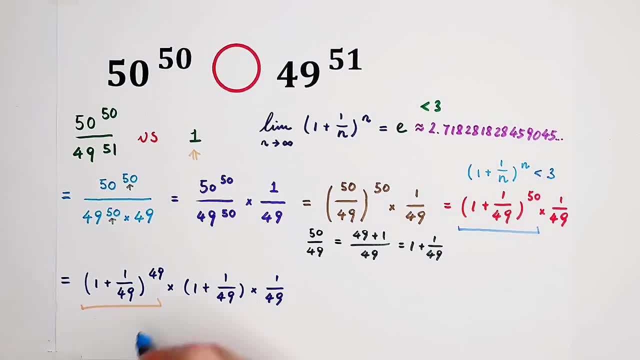 It is always smaller than 3.. So this part, it is smaller than 3.. So our last step: it is, of course, smaller than 3. times 1 plus 1 over 49 is equal to 50 over 49. And then times 1 over 49.. 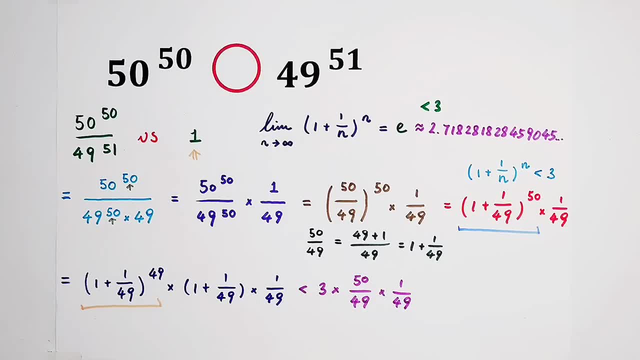 10 times 1 over 49. Calculate, calculate. Now I'm going to remind you, please don't calculate 50 over 49, it is greater than 1.. This is not the thing that we should work with. 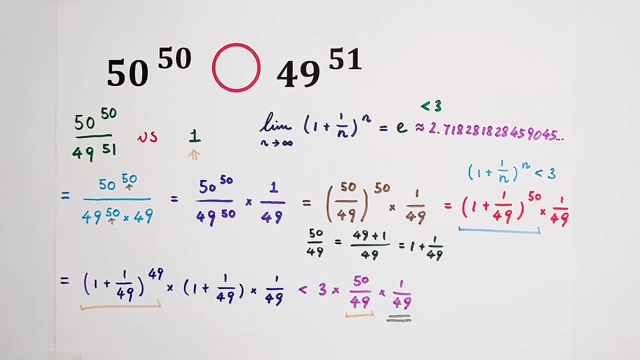 But this one, 1 over 49. It is smaller than 1 over 6.. I'm going to say, of course, obviously, For 49,, 6 are both the denominators And 49 is greater than 6.. 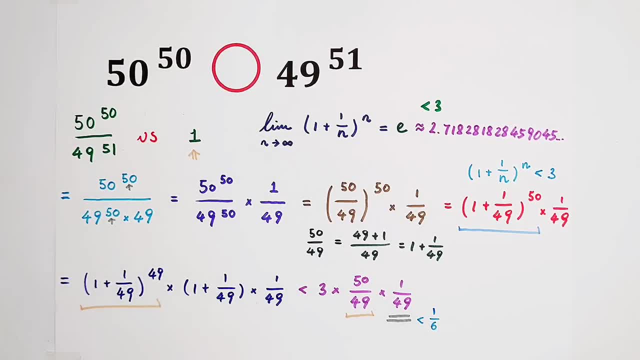 So 1 over 49 is less than 1 over 6.. Very good, In the end it is smaller than 3 times 50 over 49, times 1 over 6.. And here you can see 3 and 6 cancel. 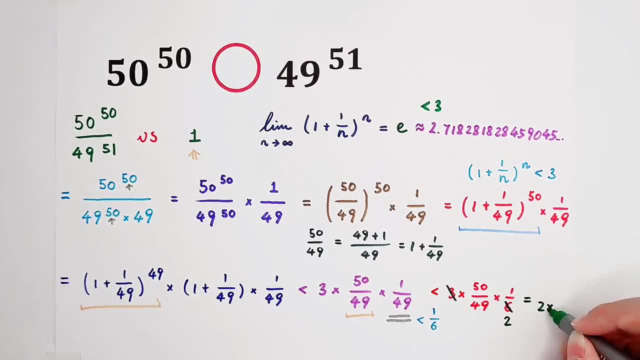 So the answer is here is 2.. 2 times 49 is the denominator And the numerator is 50. And this answer, 50 over 2 times 49, is equal to 50 over 98. So the answer is, of course, smaller than 1.. 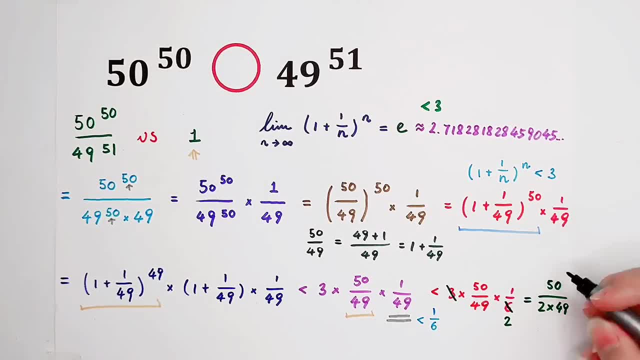 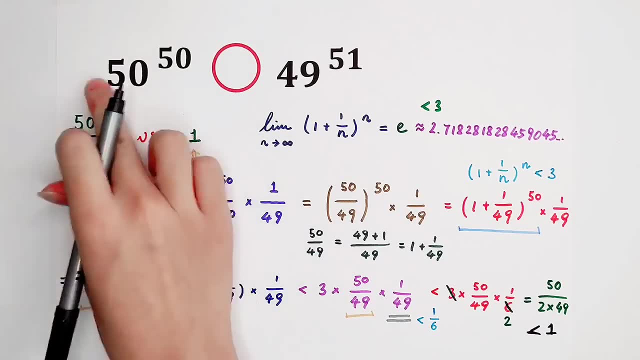 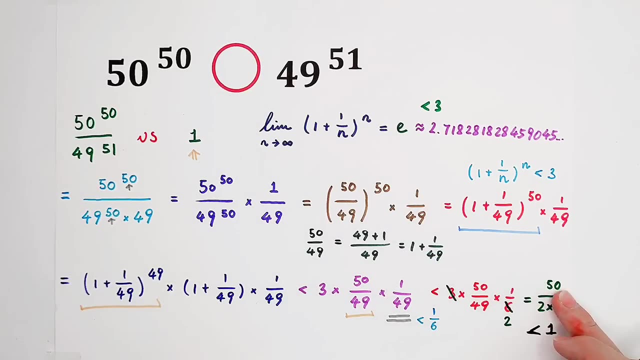 The answer is smaller than 1.. These five terms, they're all equal to the left-hand side, And the left-hand side is smaller than this, smaller than this, which is equal to this, and smaller than 1.. Here is smaller. 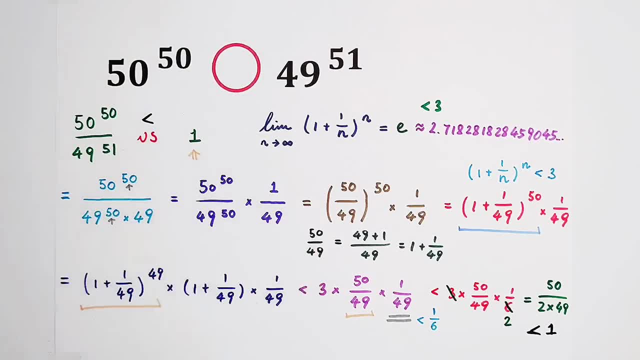 The left-hand side is less than the right-hand side. So here, if you multiply the both-hand sides by 49 times 51, we can get: the right-hand side is 49 to the power of 51.. The left-hand side is 50 to the power of 50..